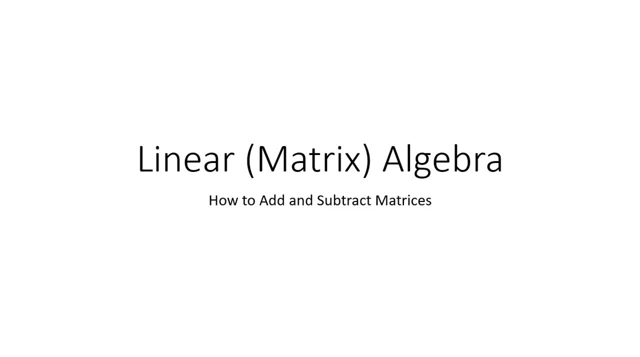 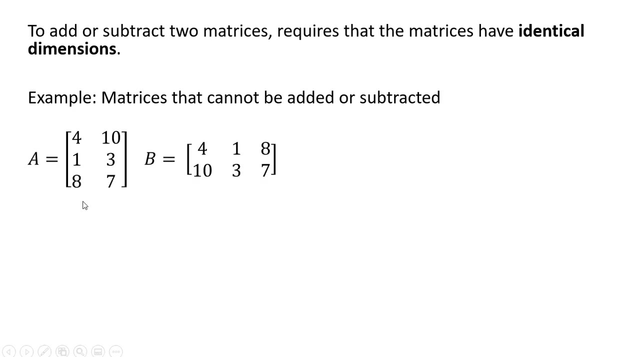 Hello, in this video we're going to look at how to add and subtract two matrices. To add or subtract two matrices requires that the matrices have identical dimensions. Matrices that cannot be added or subtracted would be these two. The dimensions differ here. This has three rows and two columns, while matrix B has two. 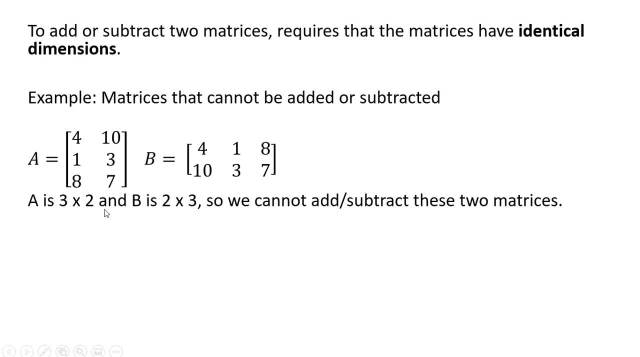 rows and three columns. So A is a 3x2 matrix, B is a 2x3 matrix. so we cannot add or subtract these two matrices. Remember, the first number refers to the number of rows, the second number refers to the number of columns. Here's another example of two matrices that cannot be added. 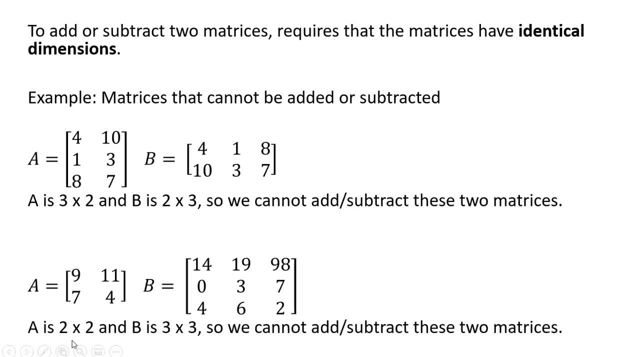 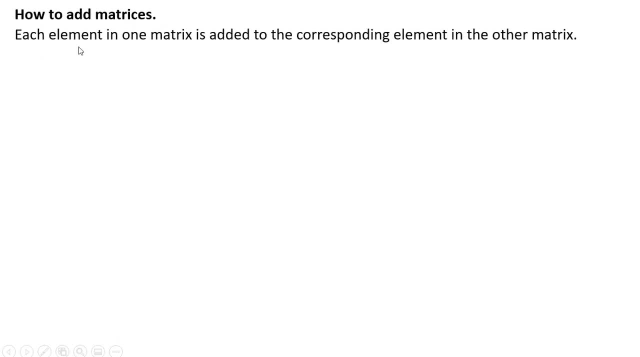 or subtracted. They differ in their dimensions. A is a 2x2 matrix, B is a 3x3 matrix. So how to add matrices? Each element in one matrix is added or subtracted. It's added to the corresponding element in the other matrix. 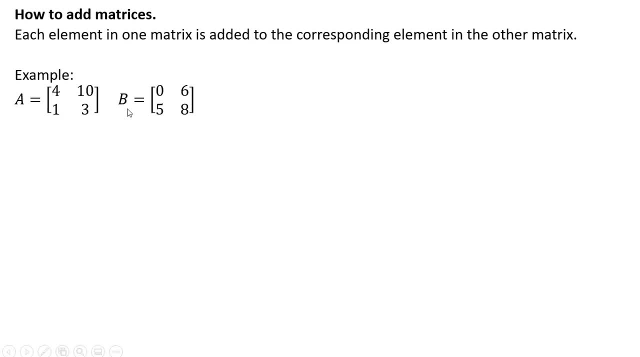 So this is how we're going to add the matrices. We've got matrix A and matrix B, so it's going to be 4 plus 0, and so I'm taking the element in one matrix and adding to it the corresponding element in the other matrix. So 4 occurs in row 1, column 1, and we're going to add to: 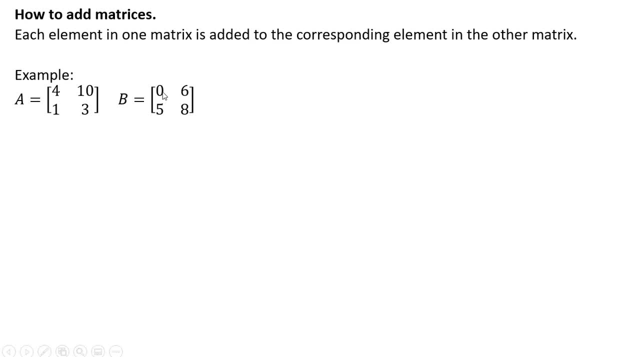 it the element in row 1, column 1 in the other matrix. Then we're going to take 10, row 1, column 2 in matrix A and add to it its corresponding element in the other matrix, row 1, column. 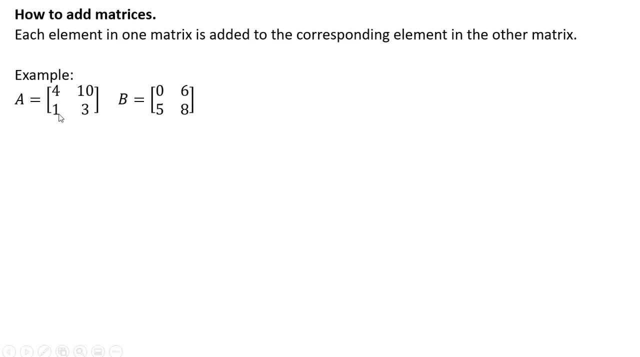 2 in matrix B. And then, likewise, we're going to take row 2, column 1 in matrix A, add to it the element in row 2, column 1 in matrix B. It's just easier to look at this visually here. so it's 4 plus 0, 10 plus 6,, 1 plus 5,, 3 plus 8, and then simplifying that. 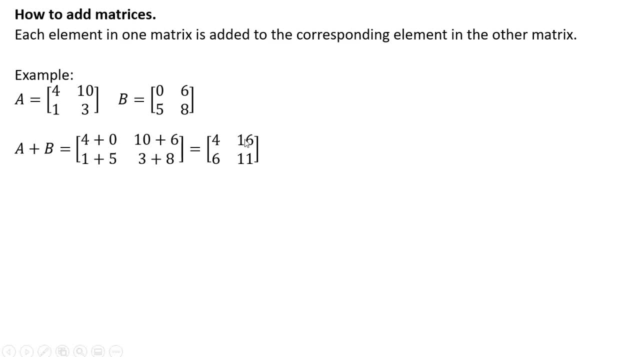 here is the result of adding matrix A and matrix B. Let's do another example. Here we have matrix A, which is a 3 by 2 matrix, and matrix B also has 3 rows, 2 columns. So 5 plus 3,, 8 plus 2, gives us our first row, 12 plus 1,, 25 plus 9, gives us our second row, 6 plus 7,, 8 plus 9,. 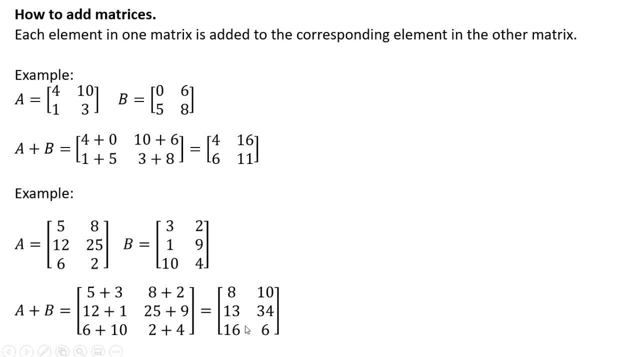 10.. 2 plus 4 gives us our third row, And then, simplifying, we have our result. All right, let's move on. How to subtract matrices. Each element in one matrix is subtracted from the corresponding element in the other matrix, So we got two 2 by 2 matrices, So it's going to be 2. 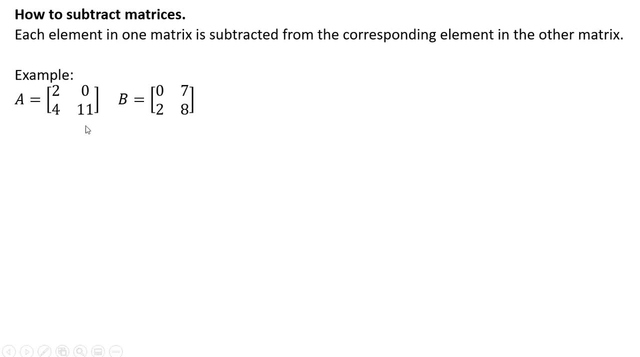 minus 0,, 0 minus 7,, 4 minus 2, and 11 minus 8.. And so here are our calculations, And here is our result of taking matrix A and subtracting from it matrix B. Let's do another example. 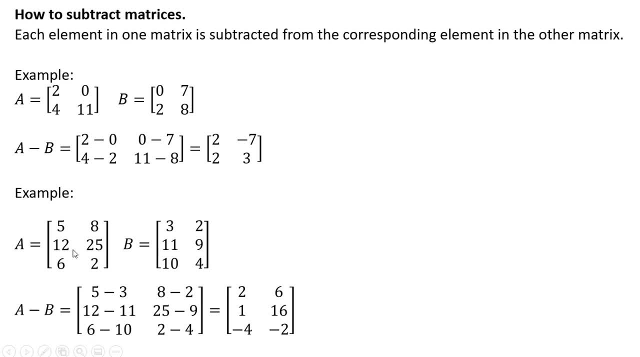 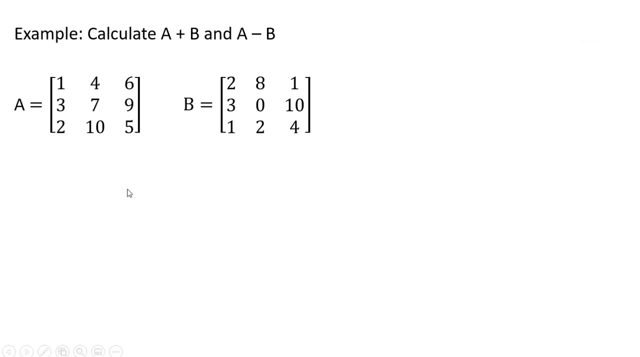 So 5 minus 3,, 8 minus 2 is our first row, 12 minus 11,, 25 minus 9 is our second row, 6 minus 10, and 2 minus 4.. Is our third row And we get the following result. Another example: We have matrix A and 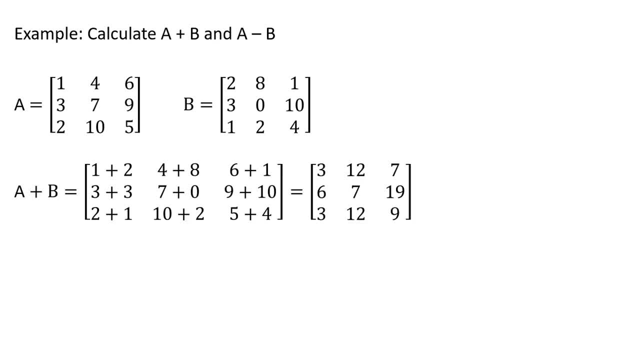 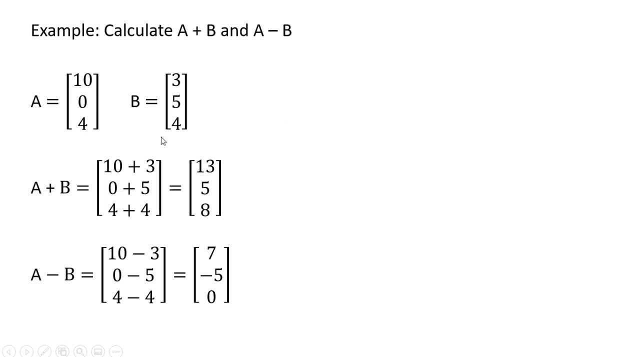 matrix B, Each are 3 by 3 matrix, And here are our calculations. And then matrix A minus matrix B gives us the following, And here's our final example: We got a column vector and column vector B 3 by 1 matrix and a 3 by 1 matrix, So we can add them And so we get the. 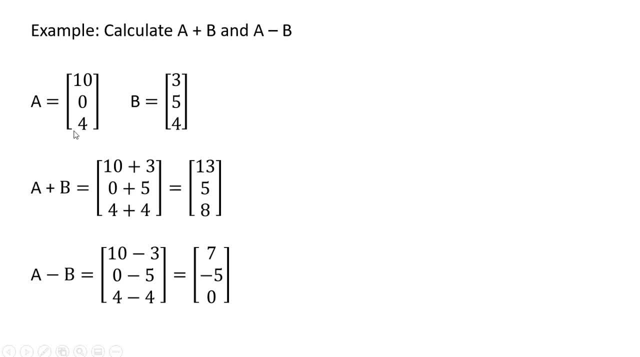 following result by adding the two matrices, And we can also subtract these matrices And we get the following result here. All right, that's it. I hope you found this video helpful.